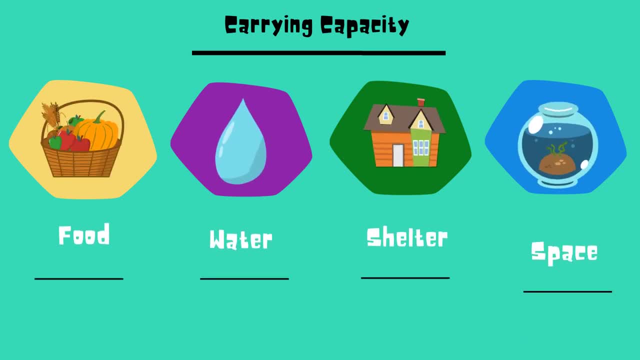 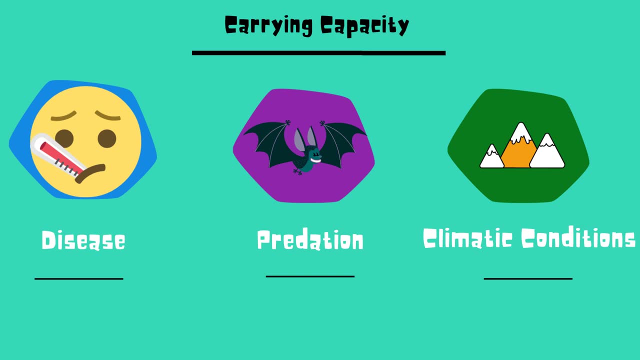 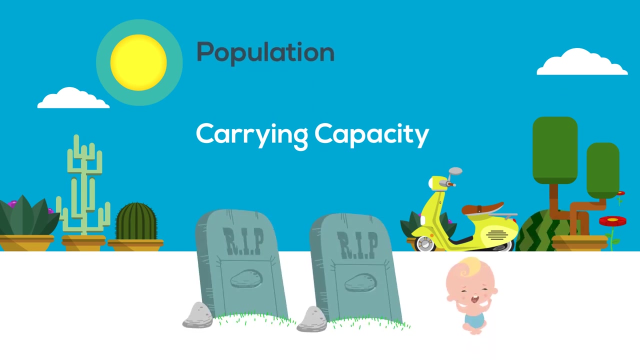 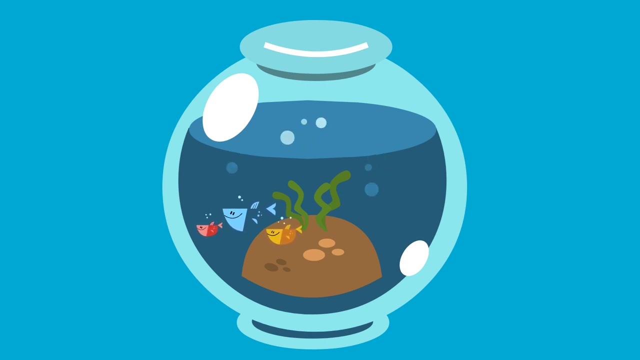 water, shelter, appropriate space, as well as disease predation and climatic conditions. If a population nears the carrying capacity, resources become limited, and if a population exceeds the carrying capacity, deaths begin to outnumber births. Let's take a look at the fish family that lives in the fish bowl. Life is plentiful, There's plenty. 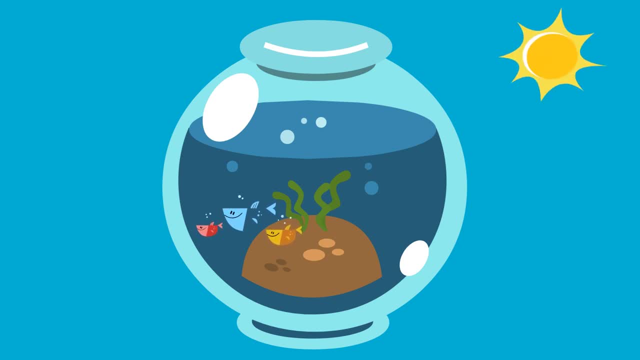 of space, there's food to eat, there's energy from the sun and they're able to reproduce rapidly. However, as they reproduce, the resources begin to become limited. They're limited by space and the amount of food. However, they're still able to reproduce Eventually. there are so many fish. 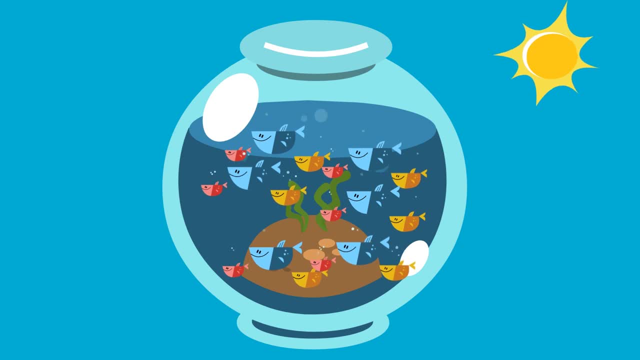 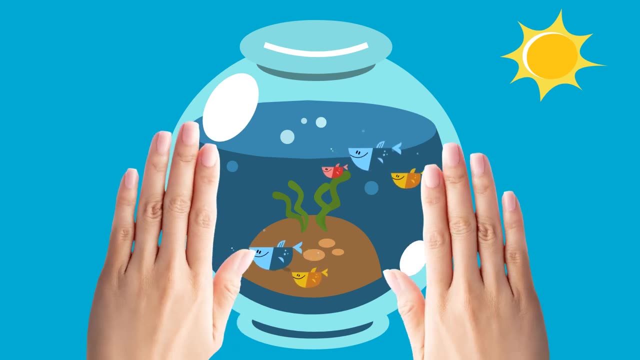 that some of the fish begin to die off because there's not food to eat and the space is limited by the size of the tank. They have reached the carrying capacity. When a population approaches its carrying capacity, the rate of increase usually slows and the birth rate equals the 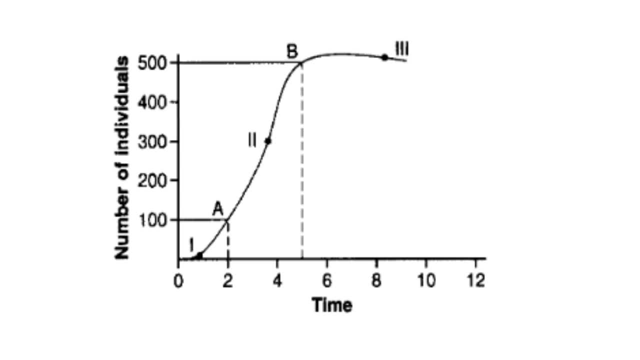 death rate. The curve plotted for this type of growth is S-shaped and shows a period of increase in growth rate, followed by leveling off as a population approaches carrying capacity. Let's take a look at the carrying capacity of a typical black bear habitat: The black bear habitat. 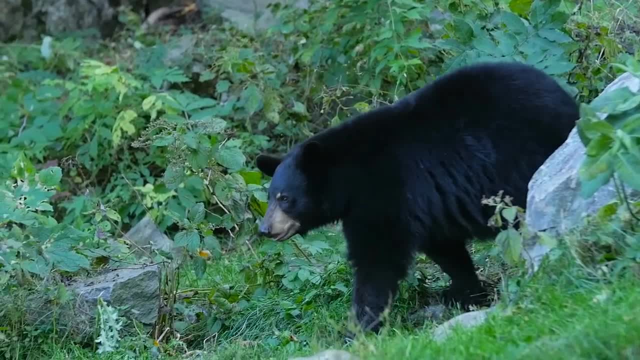 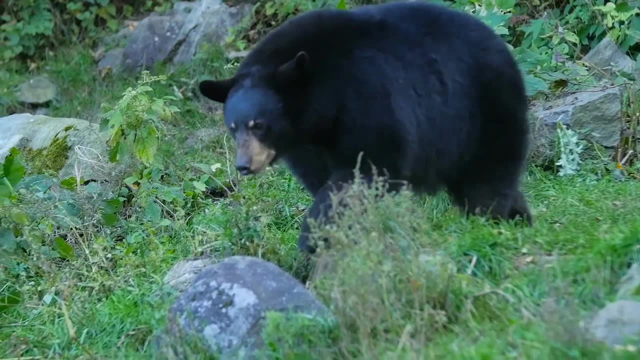 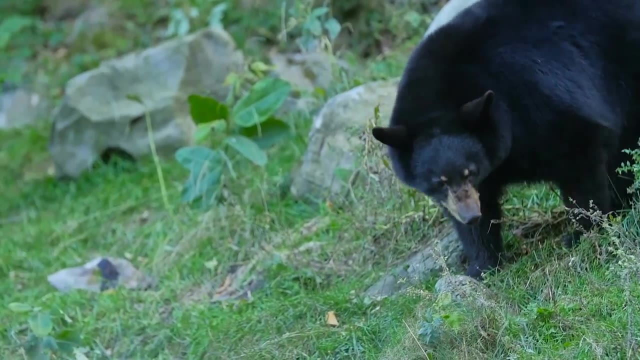 limits black bear population. The black bear habitat is a population that is limited by the through the influences of shelter, food supply and social tolerances of the species. Shelter, or cover, is a prime factor. Black bears need cover for feeding, hiding, bedding, traveling and raising cubs. 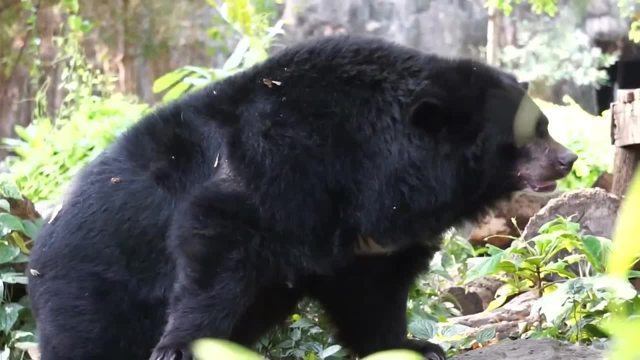 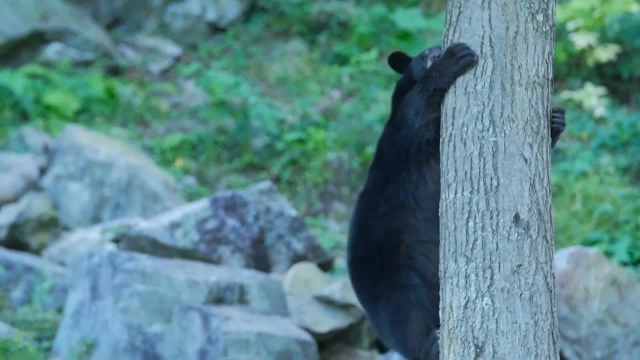 With limits of space, adult bears will kill young bears or run them out of an area. These young bears must keep moving around, either until they die or until they find an area vacated by the death of an adult. When food supplies are reduced by competition, it becomes very intense. 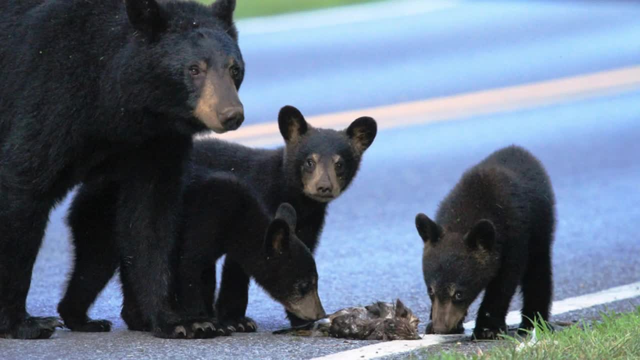 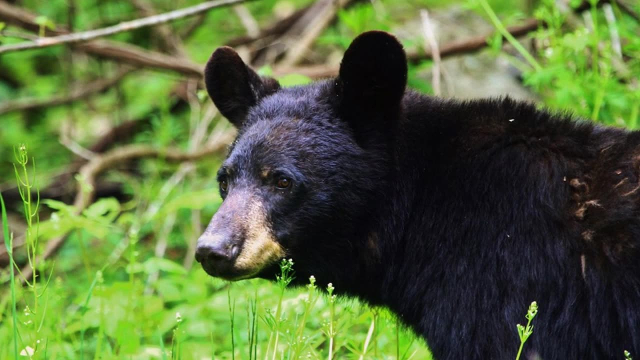 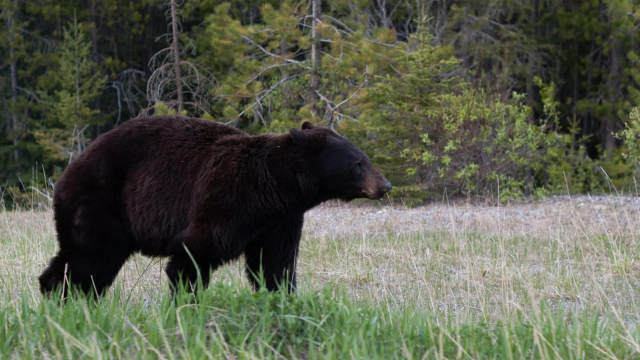 Some adult bears might temporarily move to seldom-used areas of their home range, and sometimes many miles away. They must live on what food is available in the area. These individuals may become thin and in poor condition for winter hibernation or, in the case of young bears, be forced from the area by more aggressive adults.